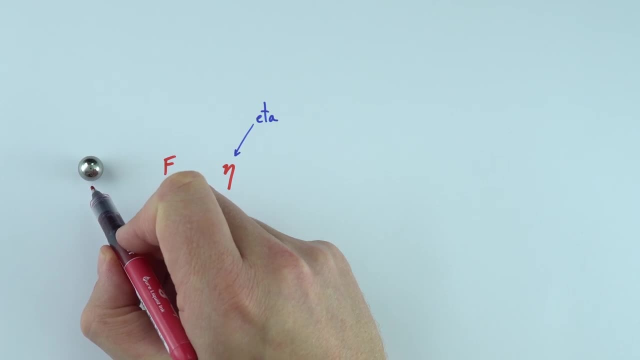 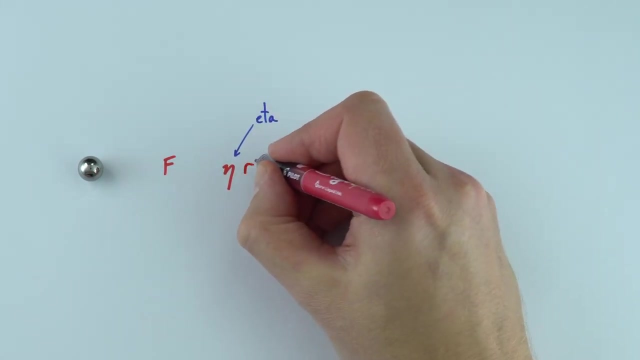 the force also depends on how big this sphere over here is. If you have something that's bigger, there's going to be a bigger surface area in contact as it's moving through that fluid and actually it's just dependent upon the radius And the other thing is it. 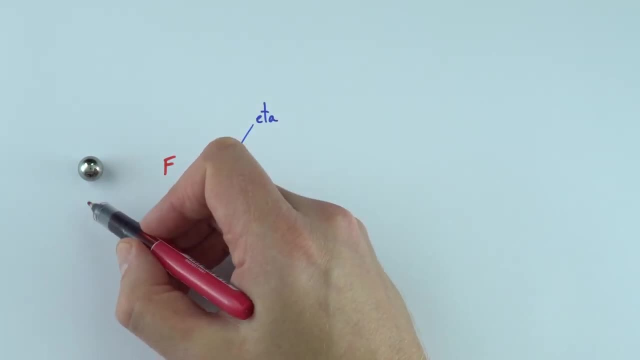 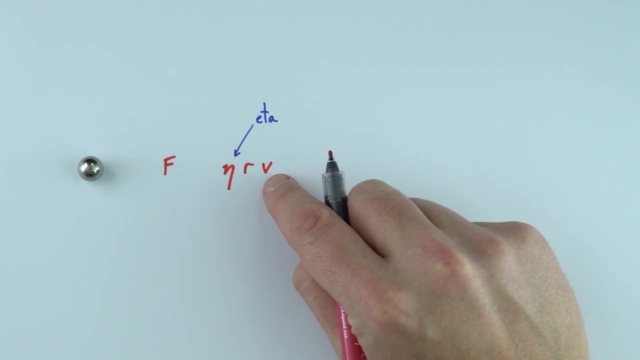 depends upon how quickly this is moving. If this is moving faster, it's going to be hitting more particles per second, so there's going to be a greater force stopping its motion. And here what we're doing is we're assuming things are moving relatively slowly, so they're 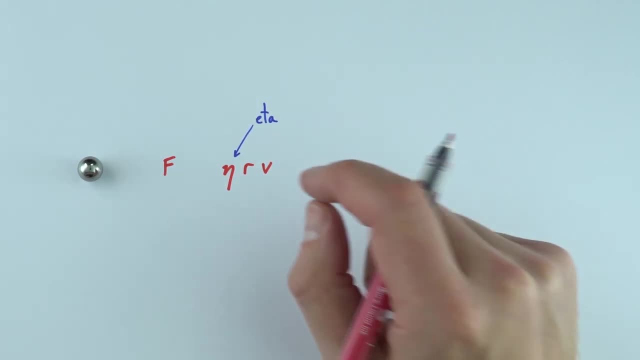 not going super, super, super fast. So this is what the force depends on, And when they did some experimentation, they found that the force was equal to equal to 6 pi eta rv. So this is Stokes' law and this tells us the size of the viscous force. 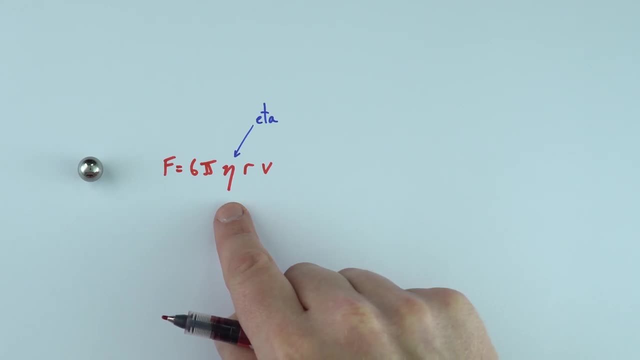 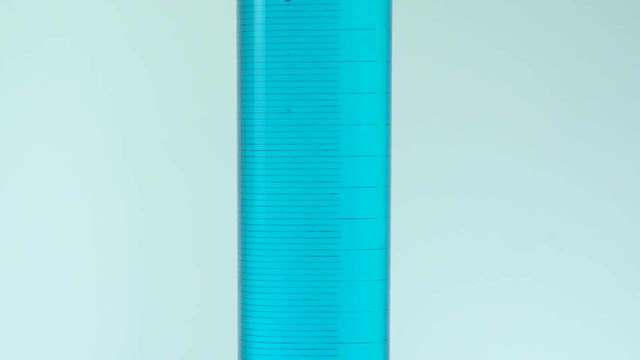 acting on a sphere as it's moving through a viscous fluid. Now let's consider the ball bearing that's falling through a liquid, like we saw at the start of this video, and let's think about the forces acting on it when it gets to terminal velocity, when it's falling at this steady speed. 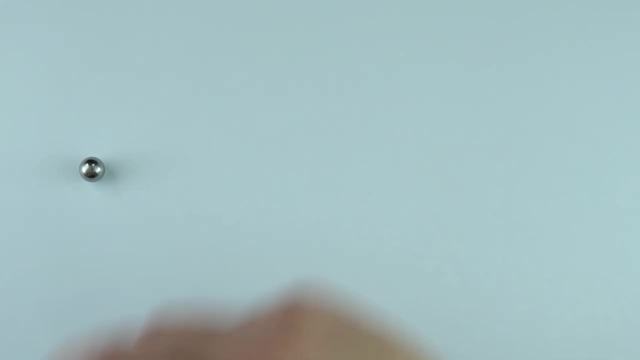 through that liquid. Now there's going to be a force upwards, due to the drag that we've just looked at, but there's also going to be a downwards force, and the downwards force is due to the weight of this object. and there's going to be one other force, and that's because there's an up thrust. 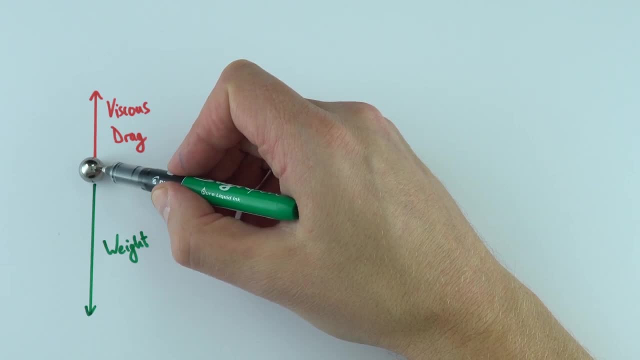 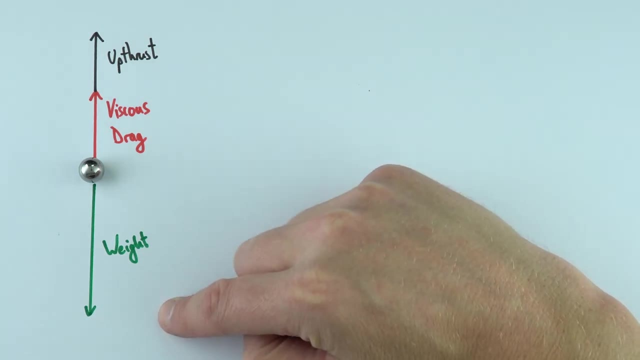 acting on this ball bearing, and this is due to the volume of fluid that it displaces. So these are the forces and, provided it's travelling at terminal velocity, we can say that the weight force down is equal to the viscous drag and the up thrust acting upwards. So I can write this: 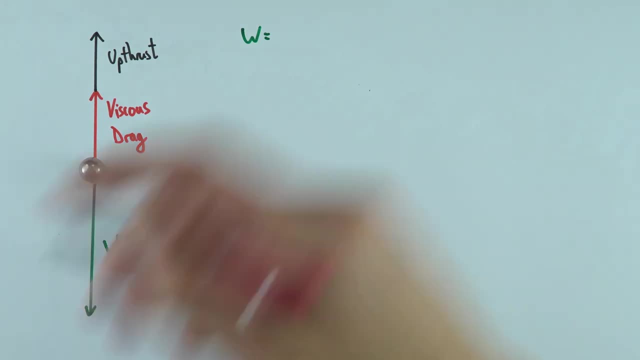 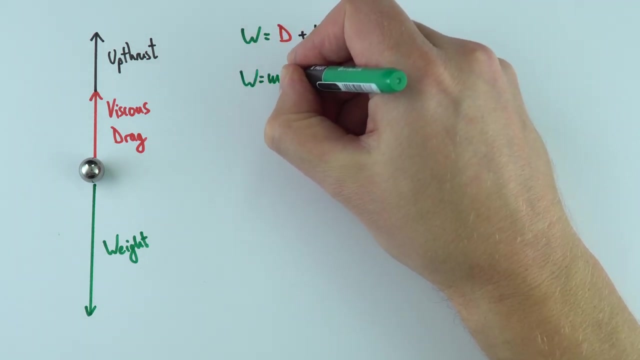 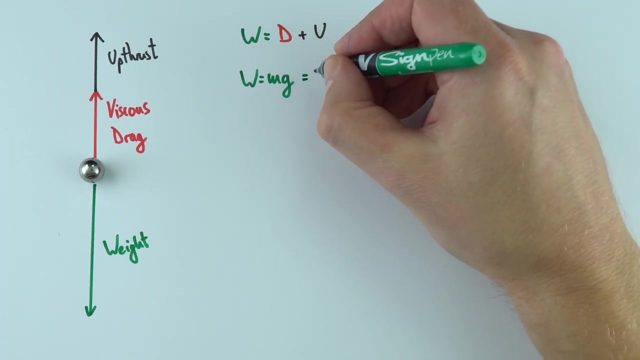 as the weight down is equal to the drag plus the up thrust. Now the weight of the object acting down is going to be equal to the mass of the ball bearing times, the gravitational field strength. but the mass is going to be equal to the density of steel multiplied by the volume. So that's going to be equal to the density of steel. 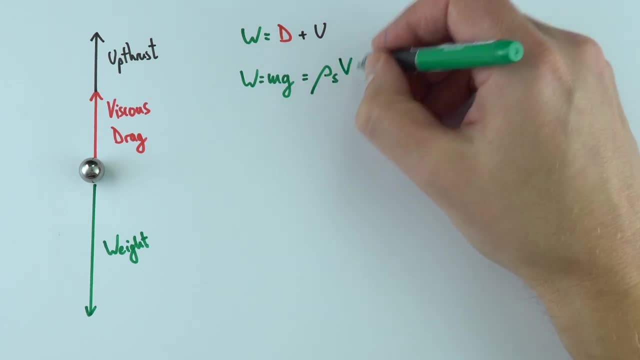 I'm going to put an s there to be my steel times, the volume times g. but the volume is equal to four thirds pi r cubed because it's a sphere. So we can also write this as rho s: four thirds pi r cubed multiplied by g. So this is an expression for the weight of the ball bearing. 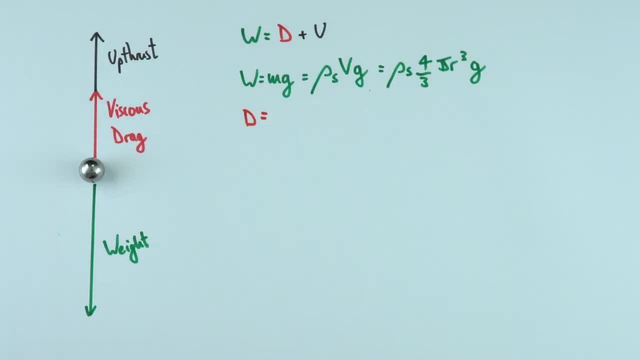 The size of the drag force, as we saw in the last part of the video, is equal to six pi, eta, r, v, and also the size of the up thrust is going to be equal to the weight of fluid displaced. Now, the weight of fluid displaced, just like we have the weight of the ball bearing up. here it now. 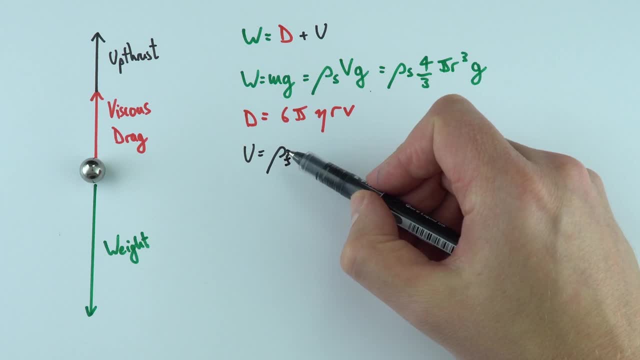 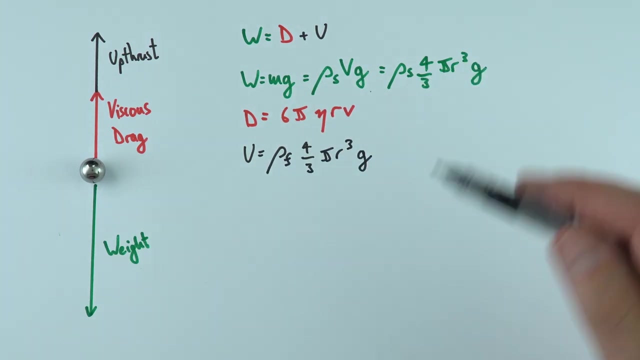 depends upon the density of that fluid. Now, that could be golden syrup, it could be water, whatever it might be. this f is just going to represent the density of that fluid. Again, it's the same volume, because it's that ball bearing so four thirds pi r cubed multiplied by g. So what I'm now going to. 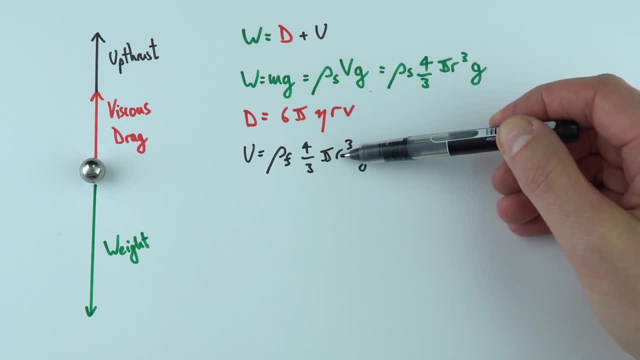 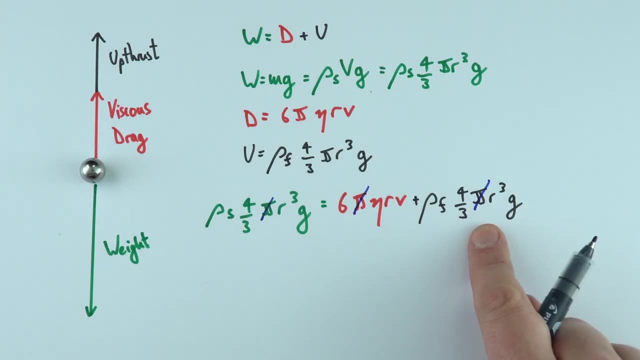 do is write this equation up here with this, this and this in it. Now, that's a lot of letters, but what we can see is there's a pi term here, here and here, so they all cancel and we've got an. 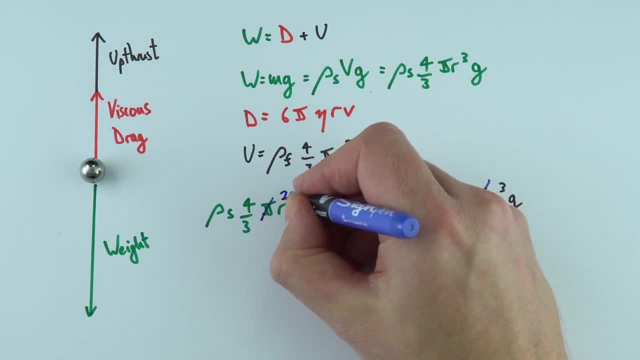 r and an r cubed. So if I take this out, that becomes r squared and this one is an r squared term as well. What I'm now going to do is just write it out again to make it a bit clearer, and we can see that six times eta, times v. so that's just this, this and this. 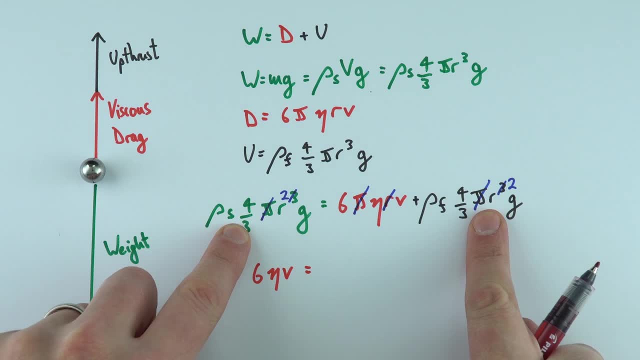 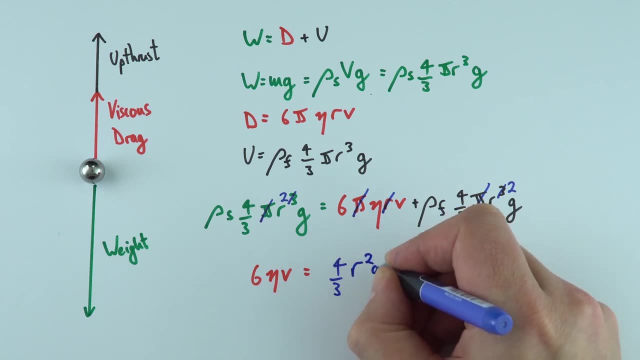 that's the same as this. take away that, And we can also write that as four thirds r squared g, multiplied by the density of s. take away the density of the fluid. So I looked at the similar terms in this and this, and then we're taking the density of this from the density of. 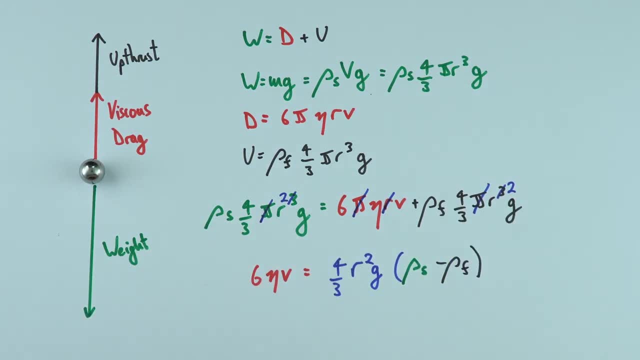 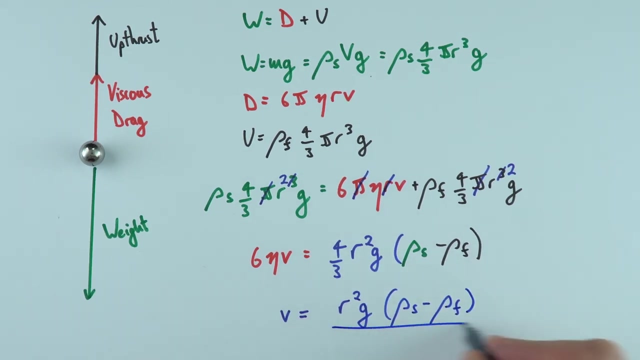 that What I can then do is I can make v the subject, So we can also write this as the v. the speed it's actually going to be travelling at is equal to r squared g of rho s minus rho f, divided by the viscosity over here Now. we've then got four over six times three. 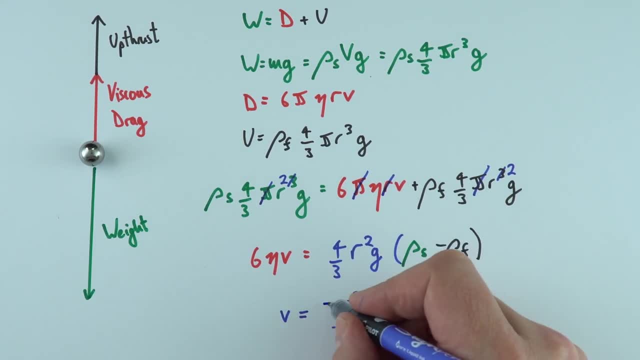 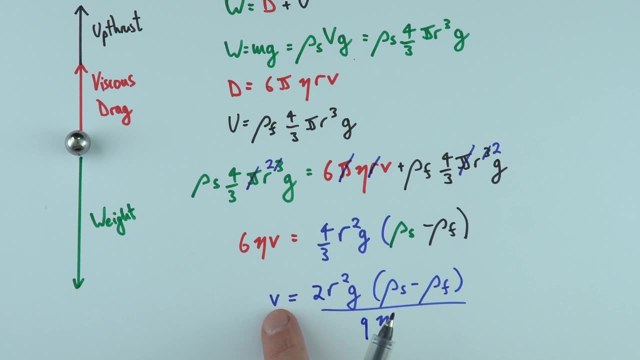 so that's the same as four over 18, which is the same as two divided by nine. Now that looks complicated, but what it's really saying is that the speed that this is going to be travelling at its terminal velocity, it depends on the size of it, and it actually depends on r squared.